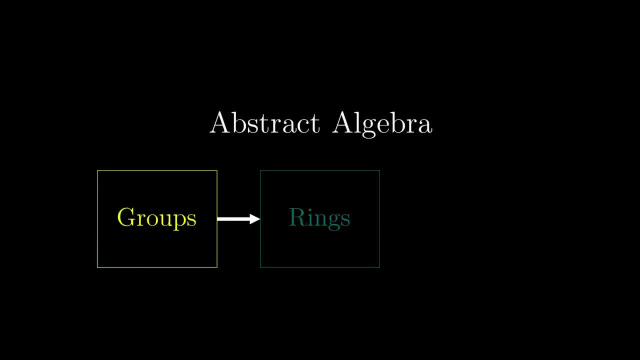 Groups are usually treated as one of the central objects in abstract algebra. Because of the word abstract, many people will struggle to see how a particular result works, But equipped with some intuitions, you might see why some theorems are blatantly true and instead say what else could. 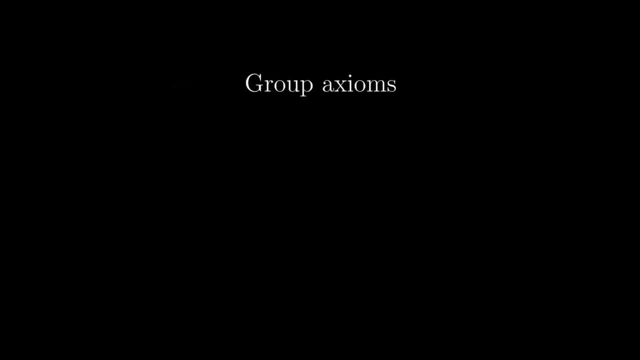 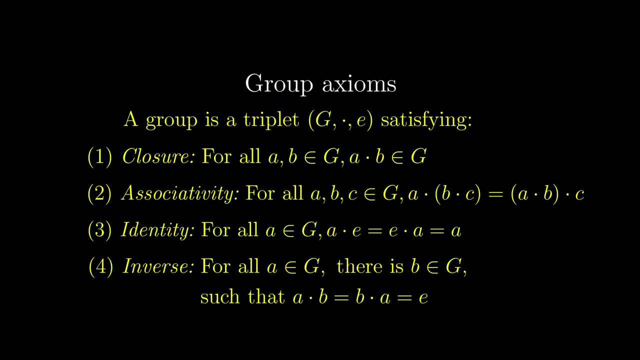 it be. Groups are mathematically defined to be something that fulfils these axioms. Although it is amazing how an entire theory is founded on these axioms, we will ignore these for now. In this video series, we will treat a group as symmetries of an object. 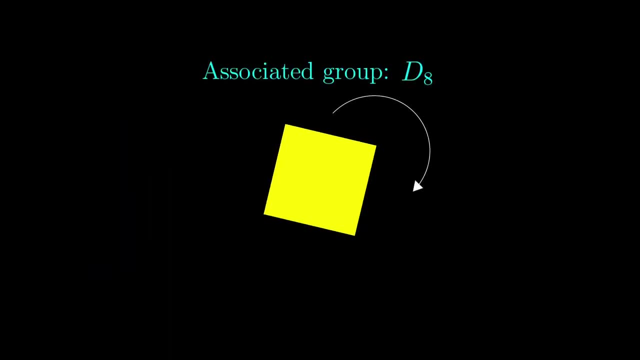 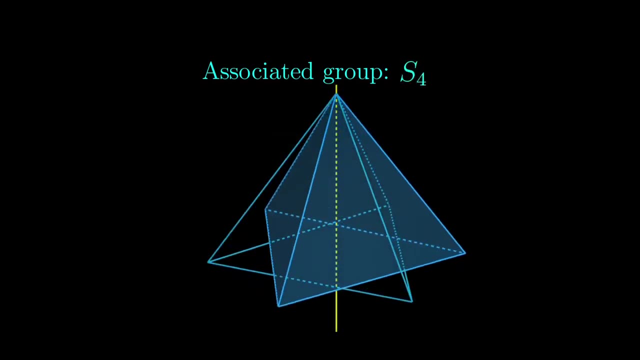 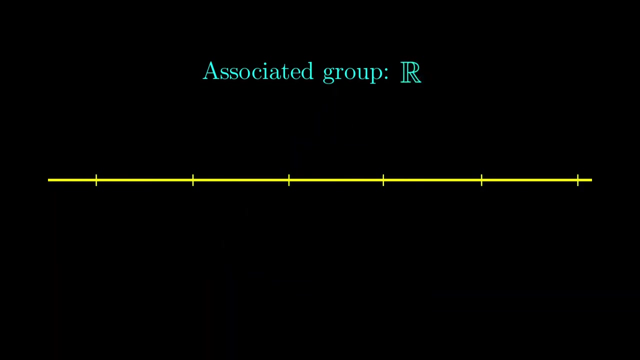 The object can be a plane figure, usually a regular polygon like a square, a solid like this regular tetrahedron, or even a real number line, Symmetries of an object- And a symmetry here means a transformation that preserves both distances and the object under. 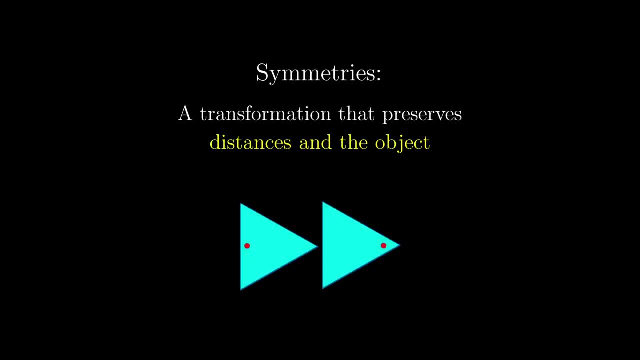 study. So this figure with two triangles doesn't have a symmetry that looks like this Because the distance between the red dots changes after the transformation. So in this case, the transformation does preserve the object, but not the object, And we are a member of the three symbols. On the other hand, 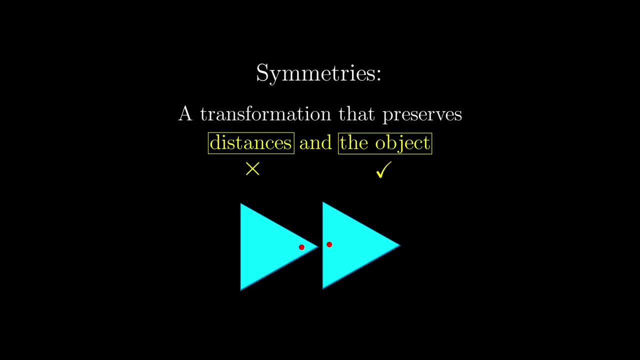 but not distances, and so it is not a symmetry of the object we are studying. When defined this way, we can see that symmetries have these kinds of properties. Namely, any composition of two symmetries is a symmetry, because all symmetries preserve: 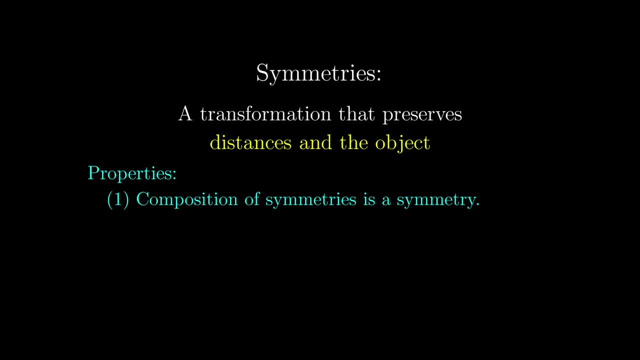 distances and the same object And compositions are associative. This means that, given ABC being symmetries, both expressions tell us to do the same symmetries in the same order. Also, not doing anything is a symmetry, because not doing anything definitely preserves distances. 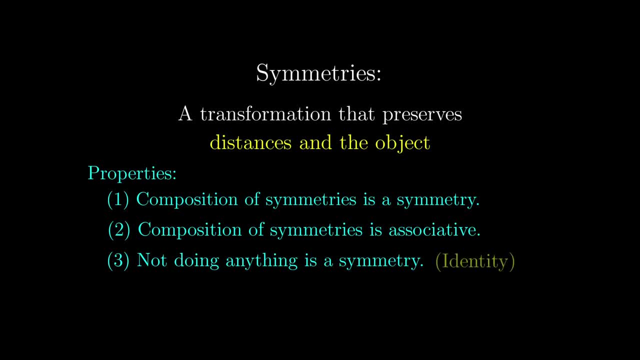 and the object. We call this symmetry of not doing anything the identity. And the last property is that we can always undo a symmetry and this symmetry will always, always be a symmetry. We will always tell that symmetry of not doing anything is the identity. 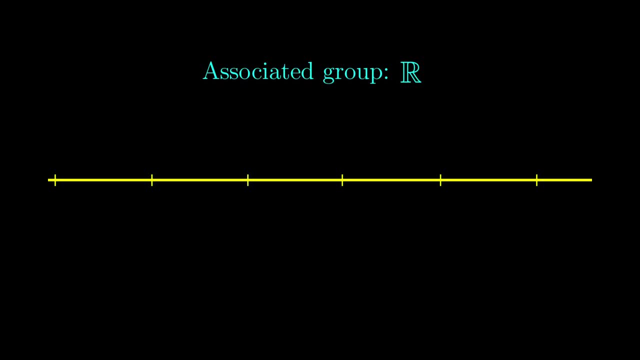 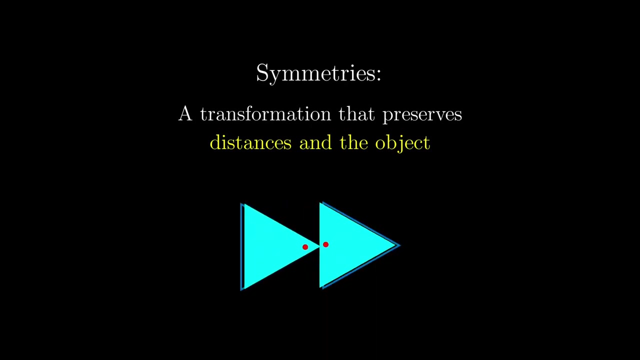 And symmetries here mean a transformation that preserves both distances and the object under study. So this figure with two triangles doesn't have a symmetry that looks like this. Because the distance between the red dots changes after the transformation. So in this case, the transformation does preserve the object. But maybe this is a performative train of thought. but not distances, and so it is not a symmetry of the object we are studying. 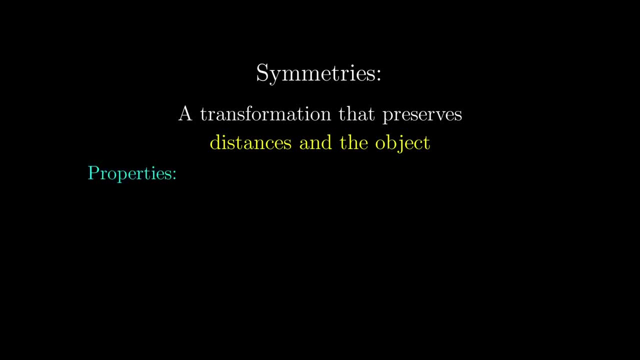 When defined this way, we can see that symmetries have these kinds of properties. Namely, any composition of two symmetries is a symmetry, because all symmetries preserve distances and the same object. And compositions are associative. This means that given A,B,C being symmetries, both expressions tell you to do the same symmetries in the same order. Also, not doing anything is a symmetry, because not doing anything definitely preserves distances and the object. We call this symmetry of not doing anything the identity. And the last property is that we can always undo a symmetry. And in this case, we must call으면 nr 2 and then чер shamu nr 1, O은 and then o yhou shuuram. And thenyor buru and thenor cur ve conform, o, c questions. And often, not because那 is not a symmetry, 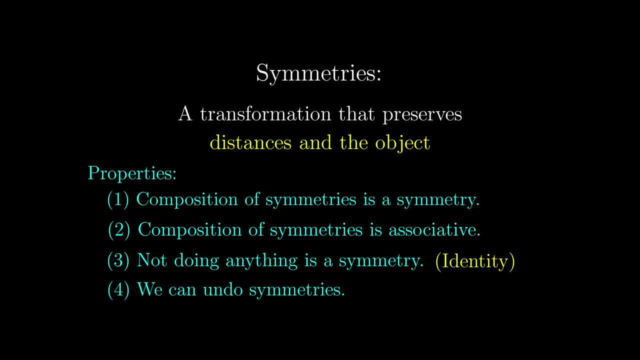 this undoing is a symmetry itself. And these four properties are what's captured in the group axioms. All these properties are pretty intuitive, and you should keep these in the 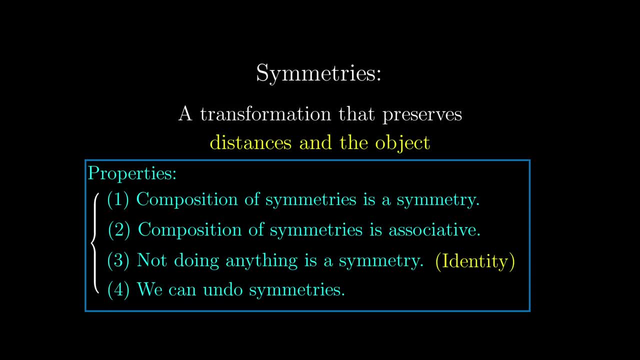 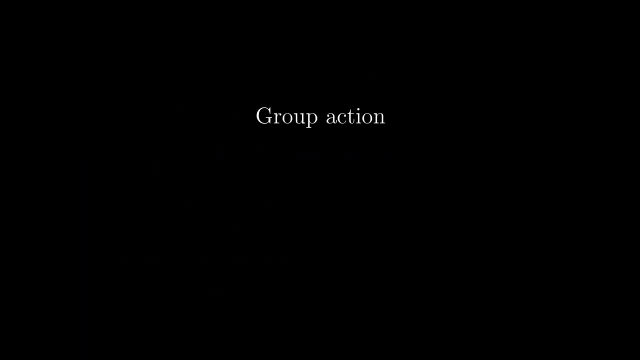 back of your mind, because we will subconsciously use them a lot of the times. Symmetries are not only useful for visualising groups themselves, but also something called group actions. Again, there are some axioms regarding what a group action is, and again, we use symmetries to visualise this concept. The key here is to see what symmetries do to the object. We usually 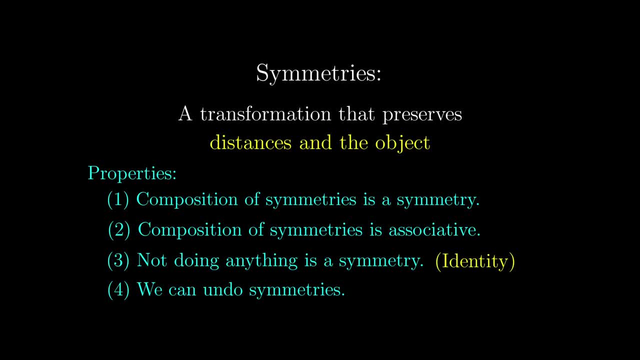 this undoing is a symmetry itself, And these four properties are what's captured in the group axioms. All these properties are pretty intuitive and you should keep these in the back of your mind because we will subconsciously use them a lot of the times. Symmetries are: 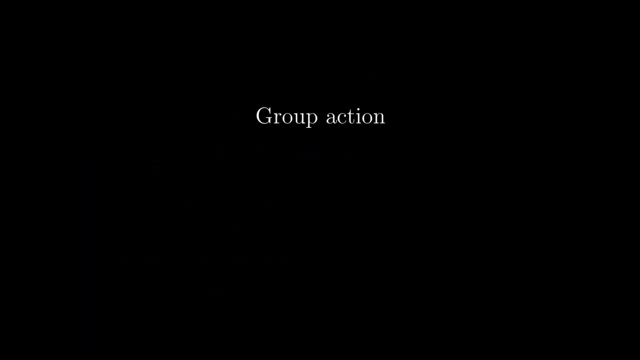 not only useful for visualising groups themselves, but also something called group actions. Again, there are some axioms regarding what a group action is, and again, we use symmetries to visualise this concept. The key here is to see what symmetries do to the object. We usually 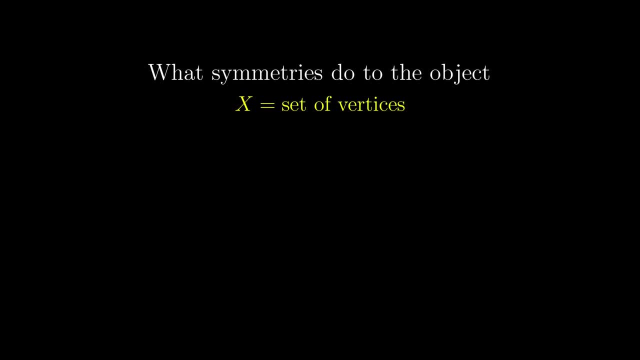 see this by only analysing what symmetries do to the vertices. For example, in this tetrahedron we label the vertices as 1,, 2,, 3 and 4.. So here we take the set x to be. 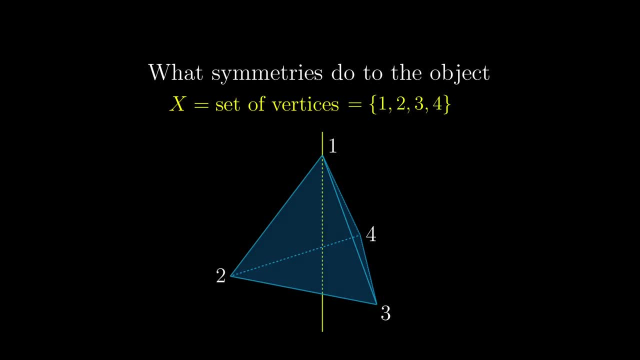 1. 1,, 2,, 3 and 4.. And notice how these vertices change under the symmetry. So now vertex 2 becomes vertex 3, which becomes vertex 4, which becomes vertex 2, under this rotational. 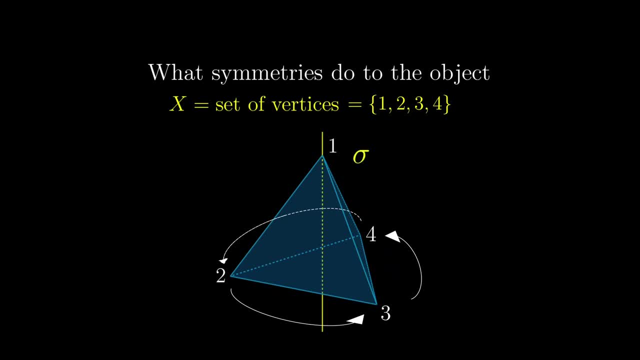 symmetry. So if we now denote this rotation as sigma, then we say that sigma star 1 equals 1. Here the star simply means that sigma star 1 equals 1.. Now of course sigma can be articulated into a set. normally The set of vertices acts. 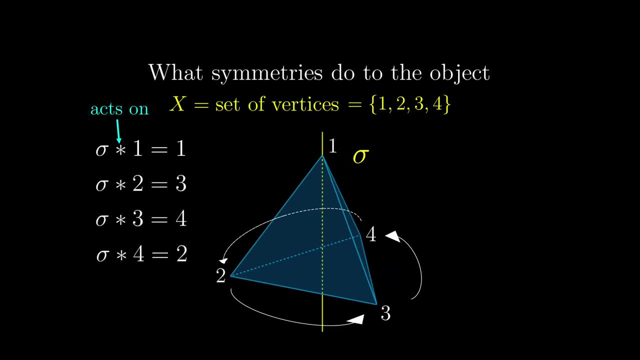 along the edges of this faces axis, corresponding to vertex 2, where the vertices also acne at the edges of this faces axis. But you can clearly see that sigma does act along the edges, along side of the vertices here And of course the set of vertices is nothing. 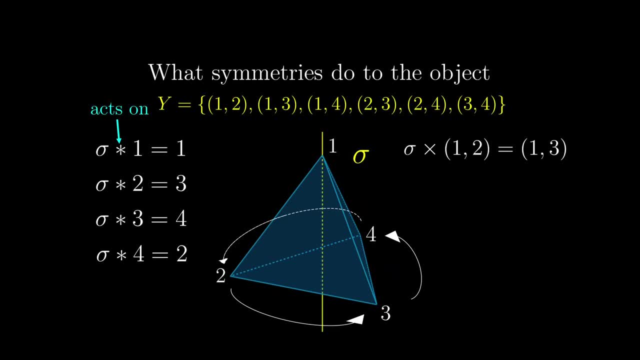 else that sigma can act on, But still it happens a lot. the cross sign has nothing to do with multiplication in the traditional sense. it just means acting on. The only thing we need to keep in mind is that when we act sigma on something in 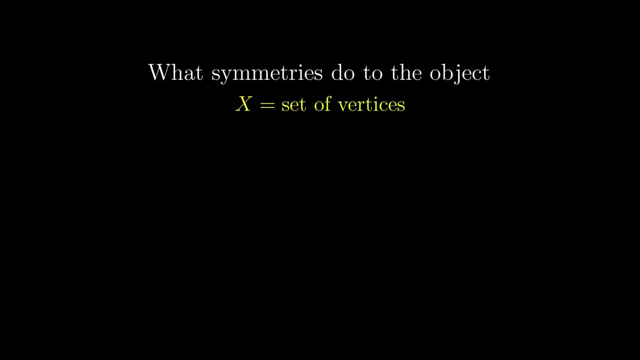 see this by only analysing what symmetries do to the vertices. For example, in this tetrahedron, we label the vertices as 1, 2, 3 and 4. So here, we take the set x to be 1. 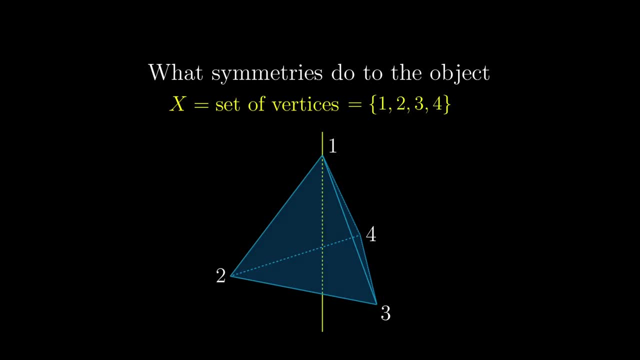 1, 2, 3 and 4. And notice how these vertices change under the symmetry. So now, vertex 2 becomes vertex 3, which becomes vertex 4, which becomes vertex 2, under this rotational symmetry. 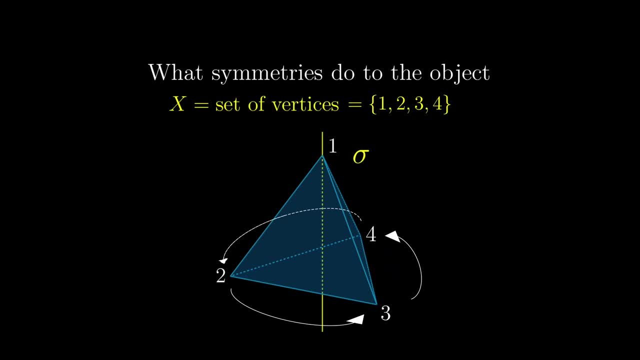 So if we now denote this rotation as sigma, then we say that sigma star 1 equals 1. Here, the star simply means that sigma star 1 equals 1. 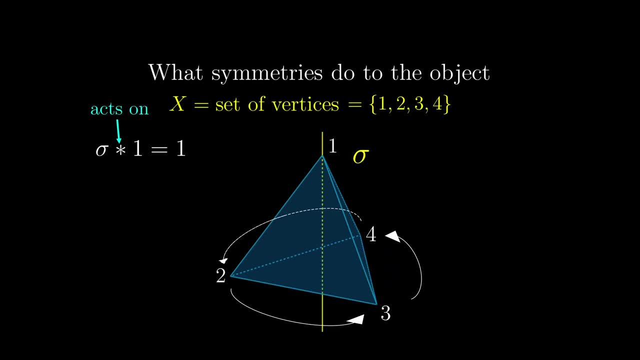 The set of vertices is not the only thing that sigma can act on. We can also consider the set of edges. Here is an example of sigma acting on the edge connecting vertices 1 and 2. Here is an example of sigma acting on the edge connecting vertices 1 and 2. And here, 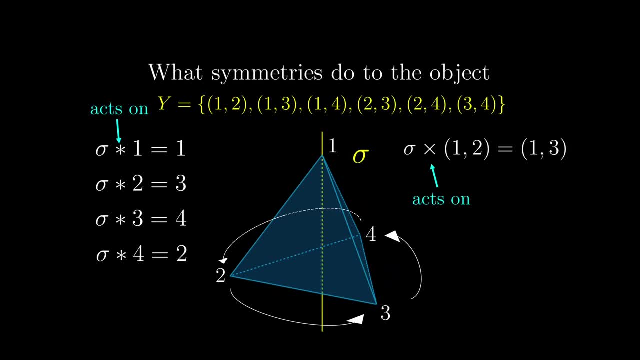 the cross sign has nothing to do with multiplication in the traditional sense. It just means acting on. 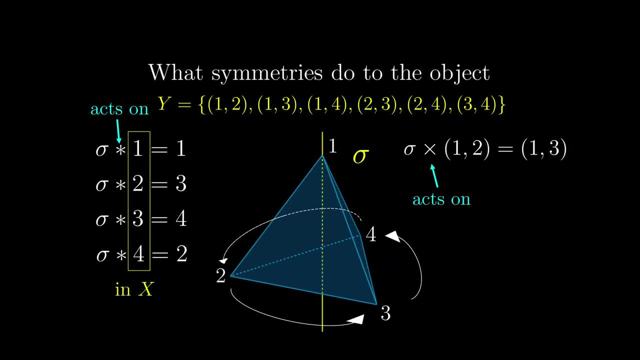 The only thing we need to keep in mind is that when we act sigma on something in the set, it outputs something in the set. And this has to be the case no matter what set 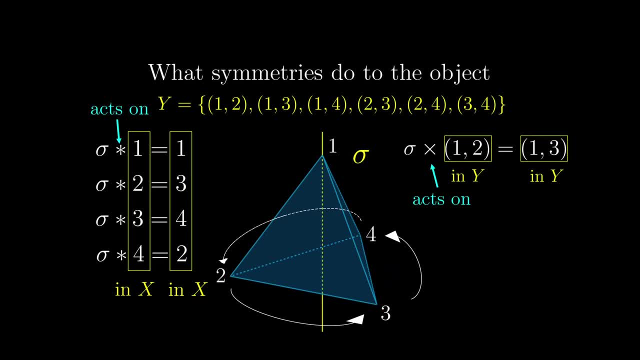 you take, which can be vertices, edges or faces. And sigma is just the set of vertices. It can be the set of vertices, edges or faces. So remember that we all define ourselves as set. Here are the symmetries. 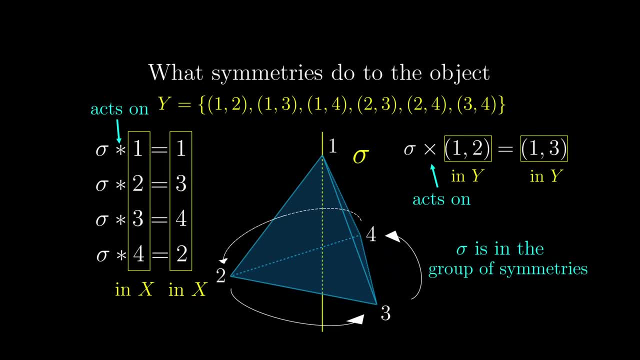 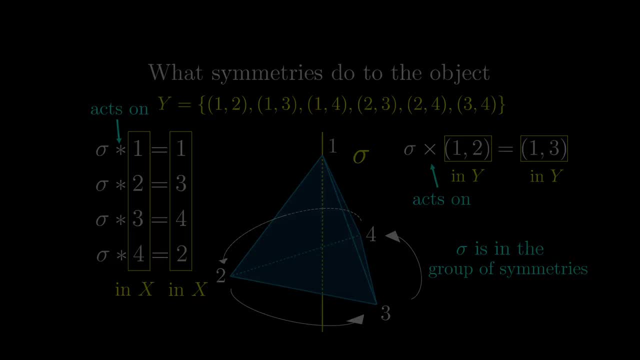 Well there is just one element in the group of symmetries of the tetrahedron. And we can define actions like what we did to sigma. So to be clear, the symmetries of an object 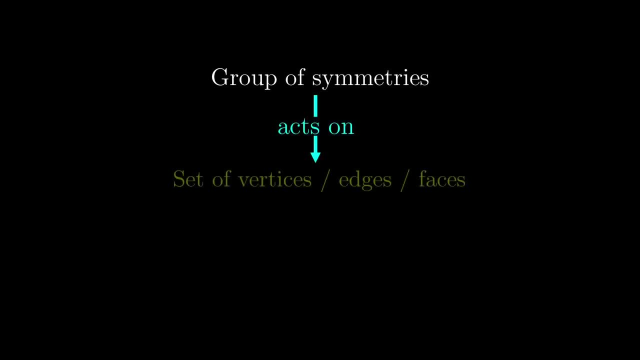 form a group, and this group acts on the set of vertices, edges or faces, to give the same set back.